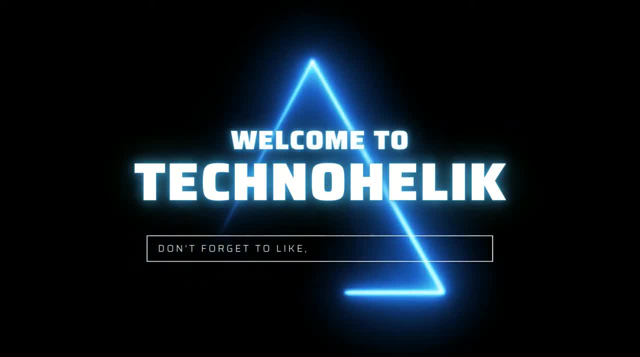 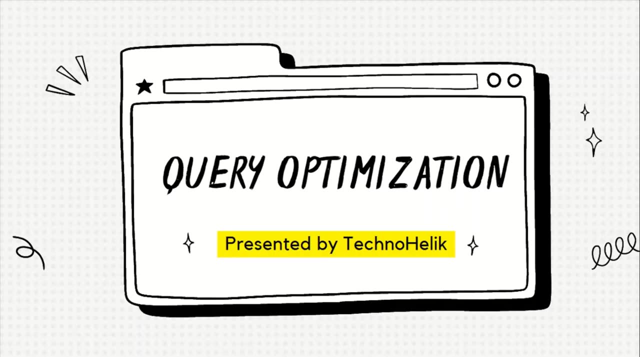 Hello friends, we know that after the huge amount of the data, we need to optimize the query for the better performance. Also, there are no rules for the how to optimize the query and improve the performance, but in this video I explain some tips for the improve the performance. 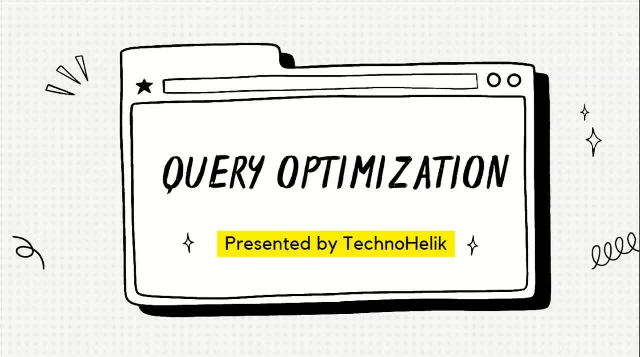 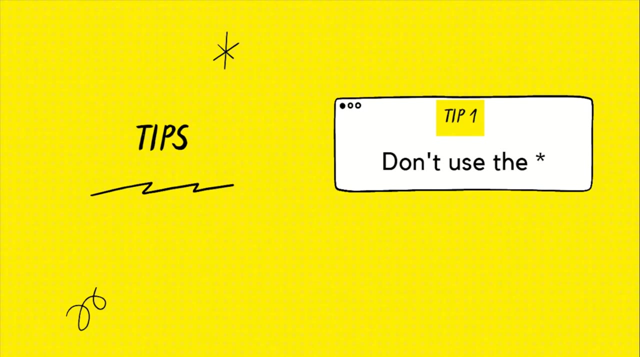 and optimize the query. I am sure these tips are more useful to you, so please watch the full video. Also, if you didn't subscribe to the channel, please subscribe to it to get the more technical videos. So let's start to get the tips, The first and most important. 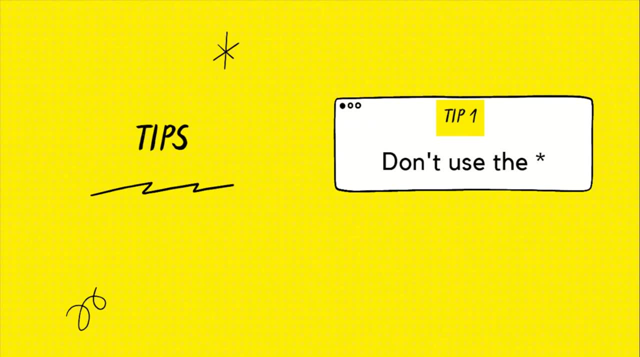 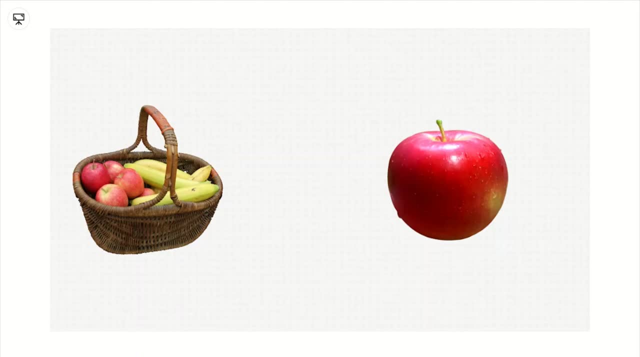 tip is: never use the star in the select query. Let's take one example. We have a one bucket which is fully filled with the different types of fruits. Now someone wants an apple Right now. what do you think to better? Take the whole basket from there and give an apple. 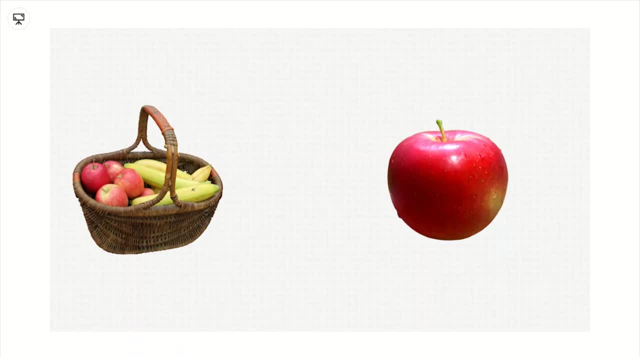 to him, or just take a single apple and give him. If you get an apple, then the apple would be a great solution. The same thing is happening with the SQL. You want some columns from the table, but you add the star in the select query. 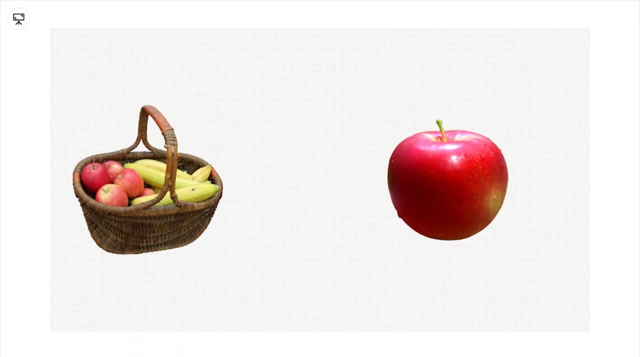 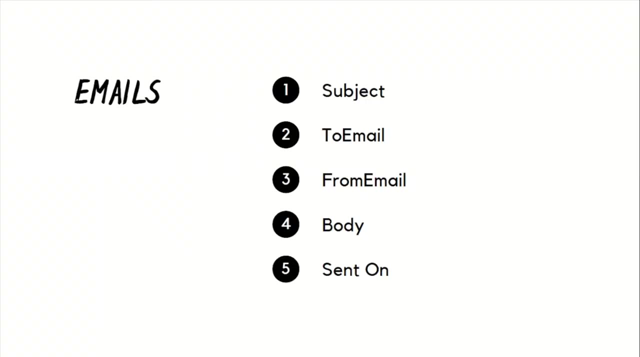 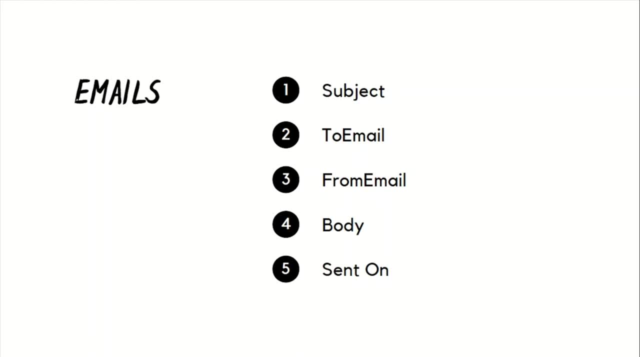 we just want the subject and email by the date filters and Silicon of Scout, but use the star. so here the body column has a huge amount of data and it takes more time to get, which is unnecessary. In short, we need to add the particular columns name, which is required. 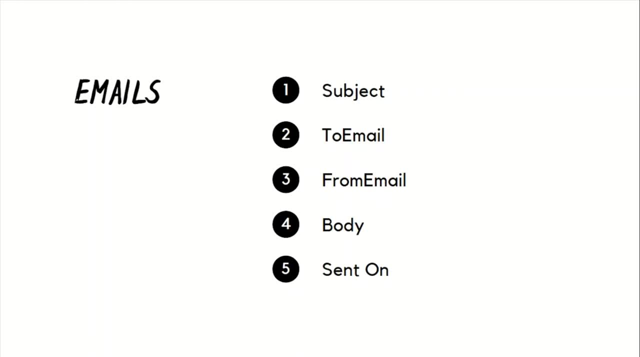 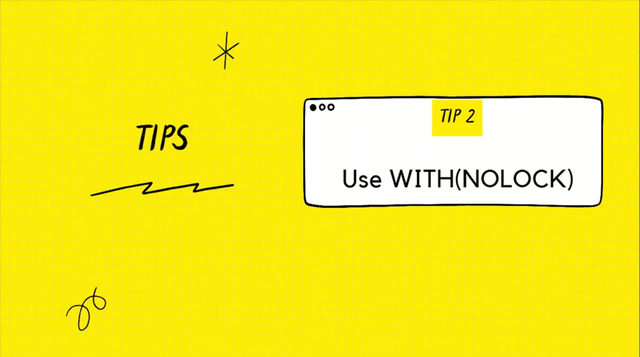 and never use the star. The second tip is to use the no lock keyword. Suppose you are on the way and someone coming from the other side Now you are waiting until he will cross to you for recognizing him. That means you are locked for a few seconds or minutes to recognize him. 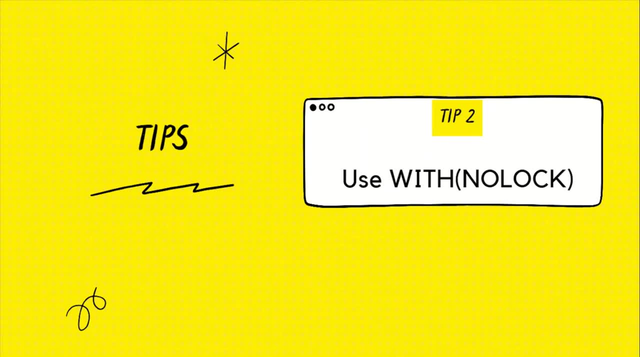 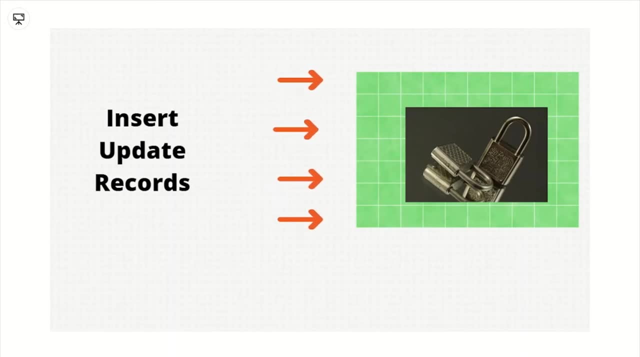 But if you ignore that person and go ahead, then you save your time. The same thing is in the SQL. when someone tries to add the insert and update the records, the table will be locked until the operation is completed. So when you try to retrieve the data, it waits for a few seconds until the table unlocks. 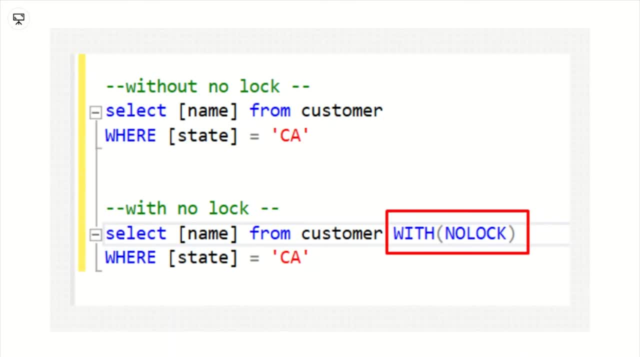 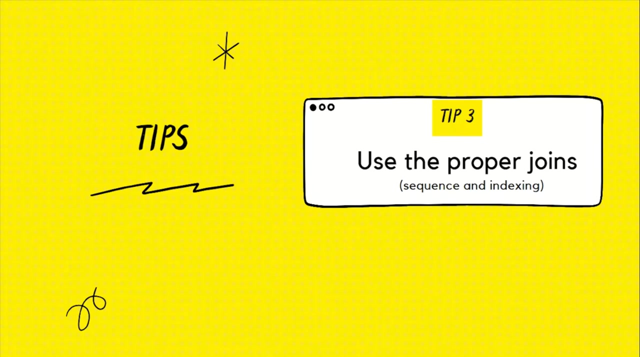 By use of the no lock keyword, you can get the data in every time and it doesn't depend on your table is locked or not. So if you don't want the real time data, you can use the with no lock syntax. The third tip is to use the proper joins. please use the proper joins. where need the inner? 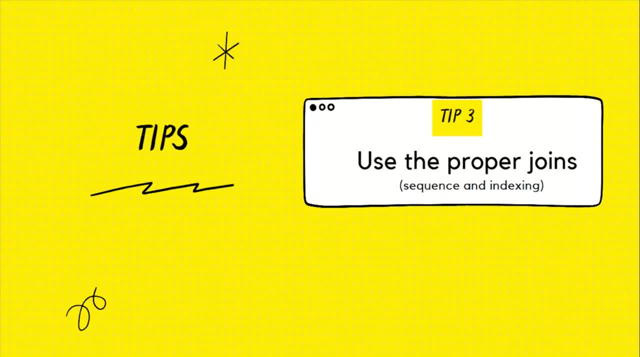 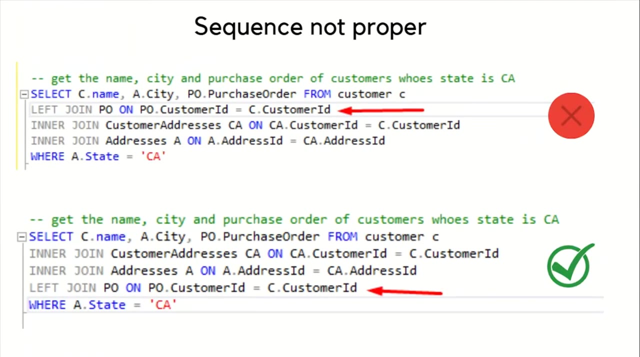 joins. don't use the left or right joins. Also, apply the proper sequence of the joins and columns according to the indexing. The sequence of the joins impact the query, So always do the joins the table with the proper sequence. In this example you can see that in the first screenshot. 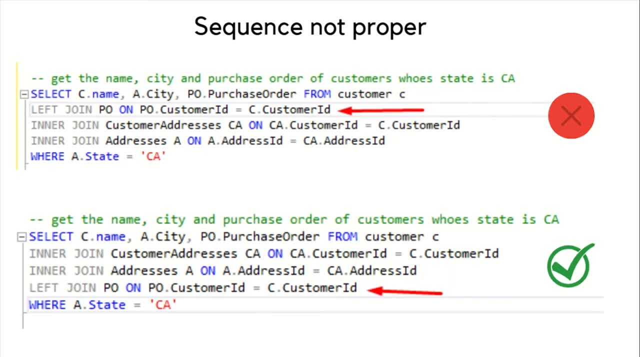 First use the left button, Left join, and then use this inner joins. It will give the proper output, but it will impact on your query performance Here. on a left join, we use all the left tables data and retrieve the match data from the right table. 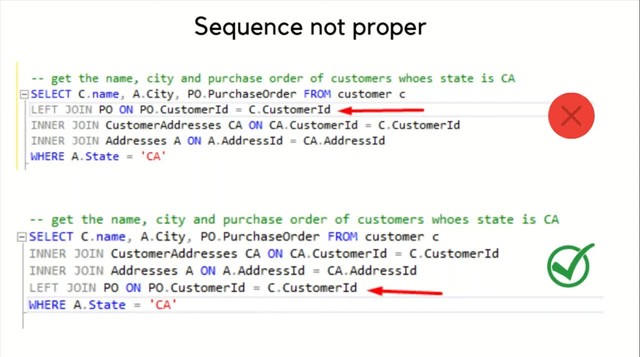 So after that we use the inner join. which means when you use the inner join, it will ignore some rows and data will be filtered. So if we use the inner joins first And then use the left join, it reduces the query time. In short, we need to use the proper sequence by the data filtering. 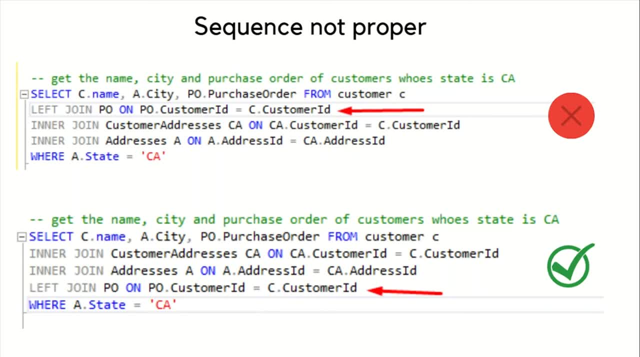 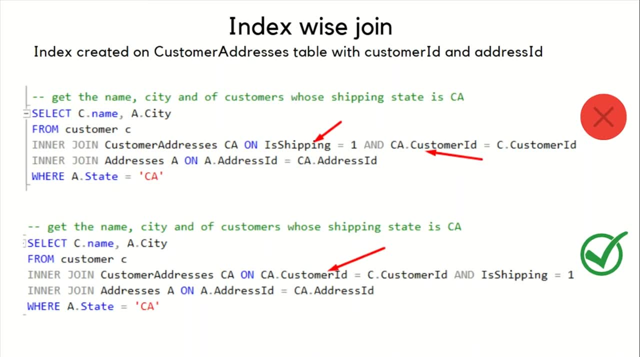 So it will reduce the joins in the row and reduce the query time. The joins column sequence also impact your query. Your joins on parameter sequence should be like this: The joins column sequence also impact your query. Your joins on parameter sequence should be like this: 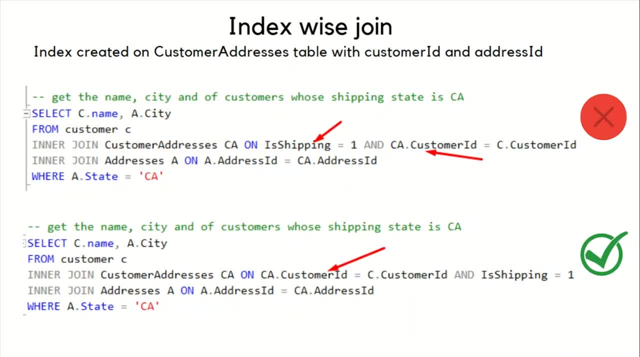 And then use the inner join, which means when you use the inner join you can check that the change are created. as per the query two. If the infrastructure changes toусer, If the script changes toこちら, So it will filter or delete. 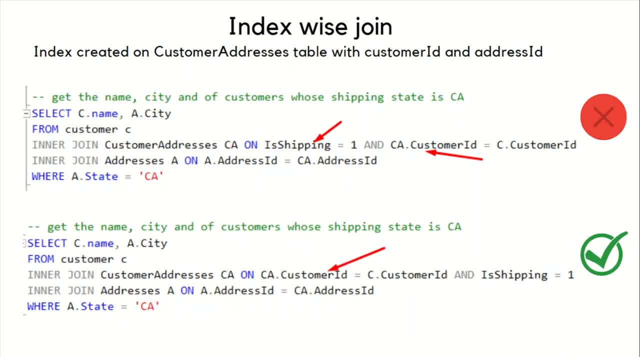 You can see here all the values of the columns shown in the hero. я significantly OK. so inside the token group I have my token in ali And then inside the every key, from here I have the token subgroup, Because from every point we will have key ablms. 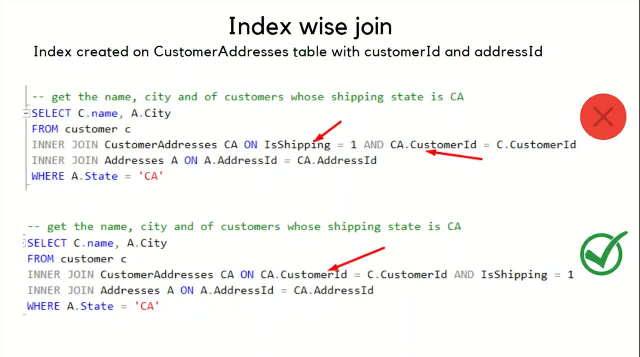 You can see here I have vengeance key in Amazon, So these are the table columns that I have selected and this canyon is my current table in Amazon address ID for the join and at the end you can use some other columns. so when you use the primary key, it will be impact or your performance when you are. 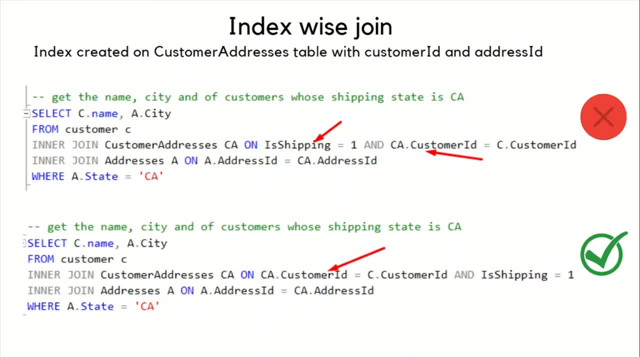 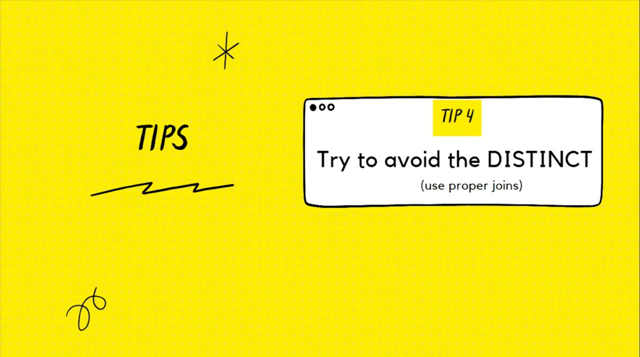 using the customer ID, it will be also impact on your performance. so if you are using, is shipping equal to one? first it will be decrease your performance. so always try to use the primary key, and then after indexing columns and then after other columns. tip number four is to try to avoid the distinct. sometimes we add some joins and 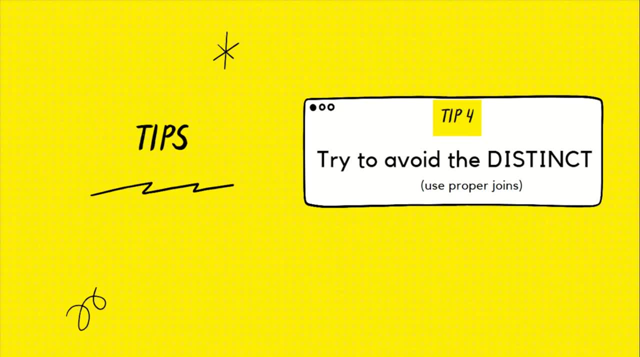 duplicate the data occurs, so that time we use the distinct keyword to ignore the duplication, but always try to find the why data is duplicated and try to solve the issue. that means always try to avoid the distinct keyword for the better performance. so this is the tip for now. 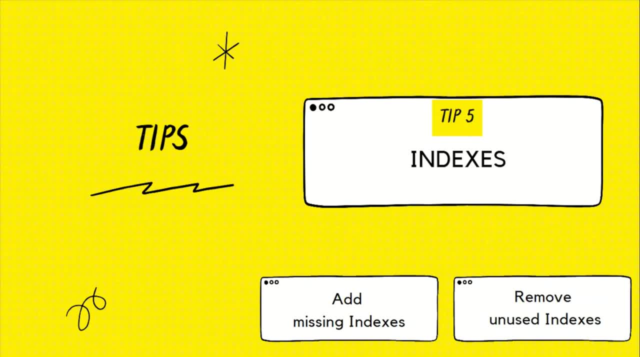 tip number five is to use a proper indexing. when you try to optimize the query, we add the missing indexing, but always check first this index: the query performance is increasing or not? also, we need to check the tables and all the sometimes we create a many indexing which are unused and it decrease the 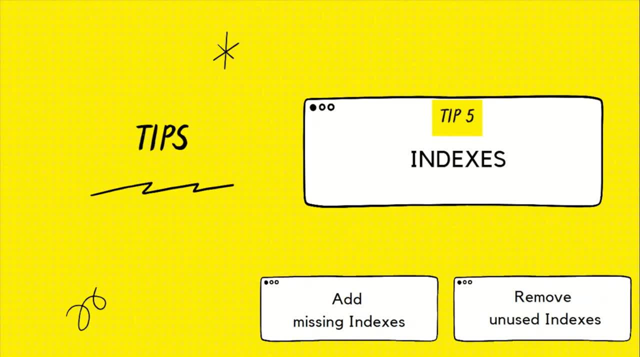 performance. therefore, please remove the unused indexing. that means please create the proper index and use the properly. tip number six is avoid to the multiple OR conditions. try to find some alternative ways if available. also, sometimes we are using the multiple OR conditions on the same column filters. let's see with this example, the first screenshot: we use the multiple OR for. 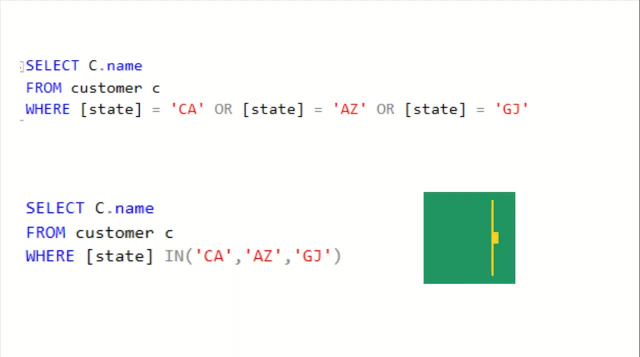 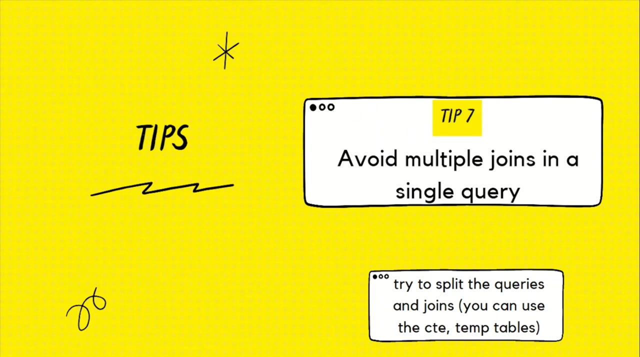 the state filter, but we can use the IN keyword for that. this change also improves your some performance, so use some alternative ways such as IN, NOT IN or etc. rather than the use of the multiple OR keywords. the next tip is to avoid too many joins in a single query, if possible, please. 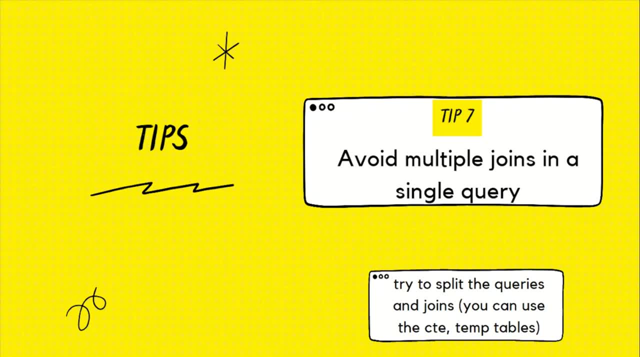 split your query into the parts. for that you can use the CTE or TAM table to avoid the too many joins in a single query. by reducing the joins you can get some improvement on your query. CEFE, number eight is the minimum use of the software is. please try to minimize. 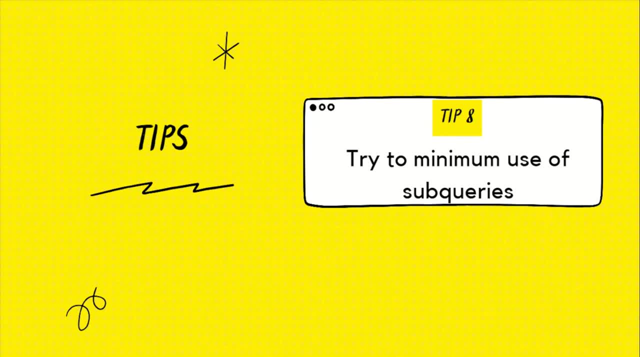 the use of the swap varies because when you use the sub query, it tries to get the data for the particular table and it takes some more time to compile and retrieve it. I am NOT saying that never use the sub query, but IF we can achieve it by the job, please try to minimize the use of the sub query, because when you use 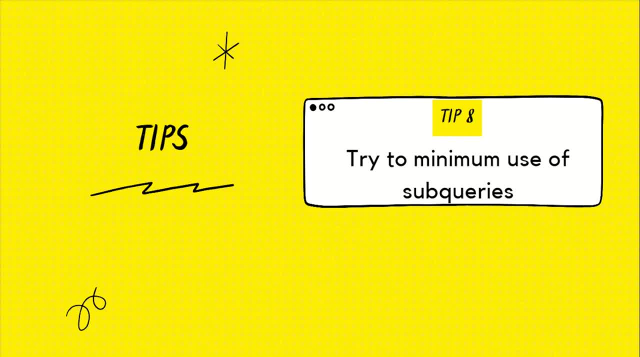 the sub query it tries to get the data for the particular table and it takes by the joins. please use that. try to avoid the sub queries in rare conditions. Tip number 9 is: use the union all rather than use of the union. The difference between the union and union all is that union all gets the all the data.